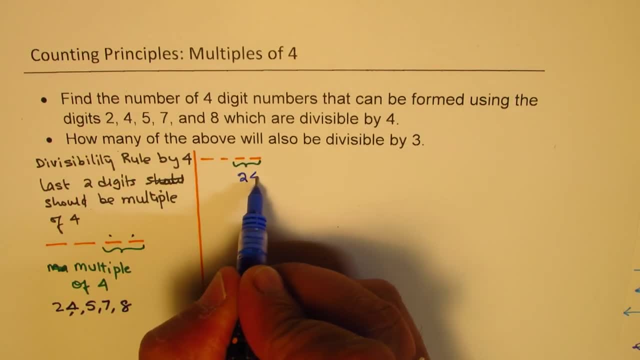 One could be 24,, for example. So 24 is a multiple of 4,. 6 times 4 is 24.. So if 24 is a multiple, 42 is also a multiple of 4, right, When you do a, 42 is not a multiple of 4, okay, 24 is okay. 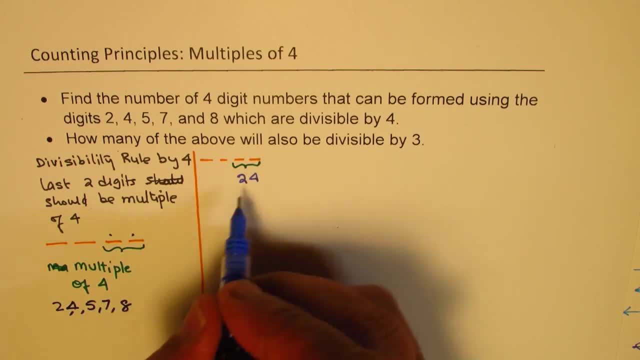 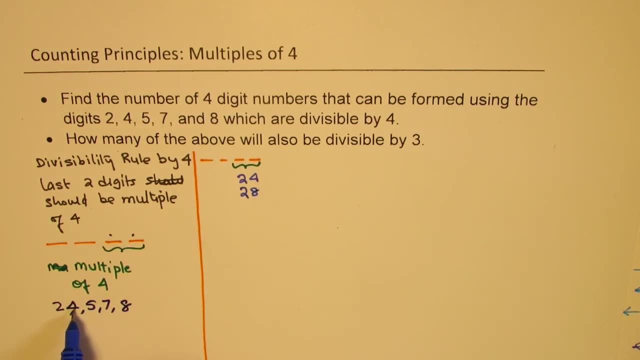 but with 2 we have 28 as a multiple right, so we have 28 as a multiple. then let's see multiples with 4. with 4, 42 is not a multiple, but 48 is a multiple right, so 48 is a multiple now with 5. 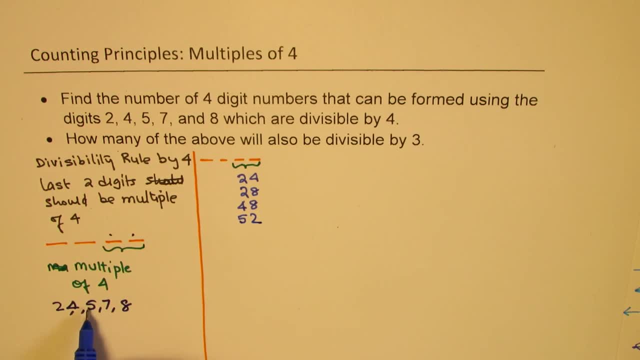 52 is a multiple. uh, 54 is not a multiple, but 58 is also not a multiple. now, with 7, 72 is a multiple of 4. 74 is not a multiple. 78, if i do 78, is also not a multiple of 4, right? 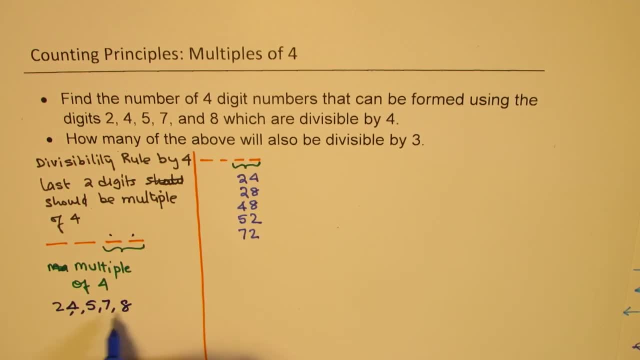 now let's look into 8. with 8, 84 is a multiple, correct. so 1, 2, 3, 4, 5, 6, so we have 6 multiples of 4. right now we have to see that if we are looking at these two, 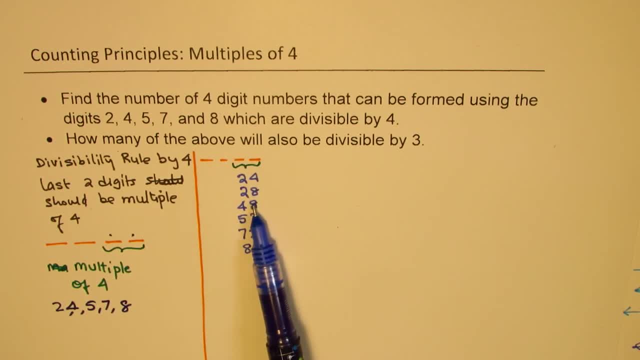 fixed on the last two positions. we have 1, 2, 3, 4, 5, 6 total combinations. now, with 24 fixed, how many numbers can be placed in these two? well, in these two we have a choice out of three right. so it could be three times two right. so those are the combinations for each which can be placed on. 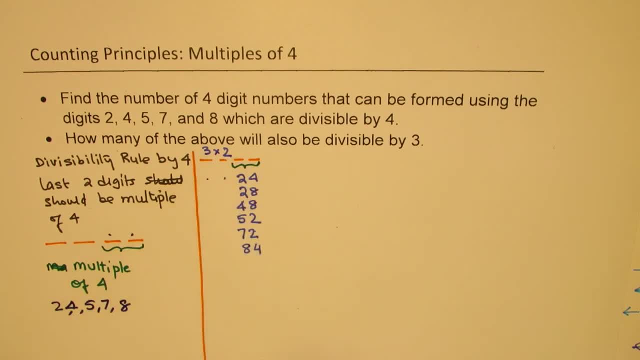 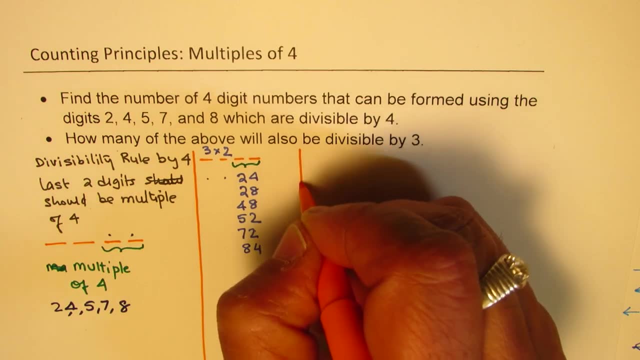 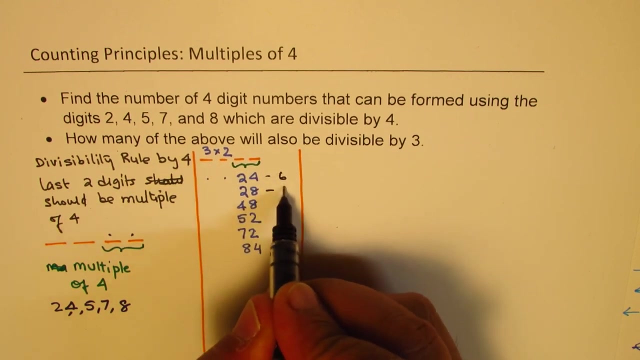 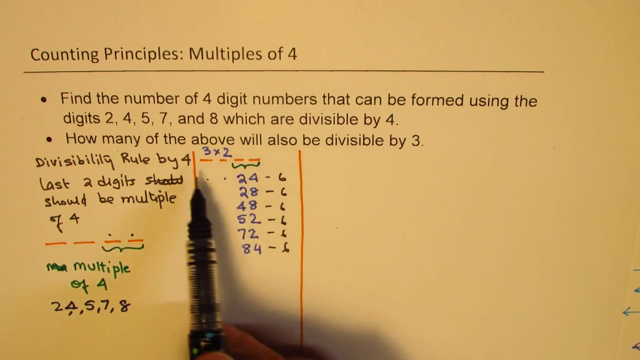 these two, once we fix the last two and you get a combination of four numbers. is that clear to you, right? so with that in mind, we can actually write down the solution for part a, and that is, for each, we get six combinations, right? so there are six numbers for each, ending with 24, 28 and so on, which are multiples of four, and 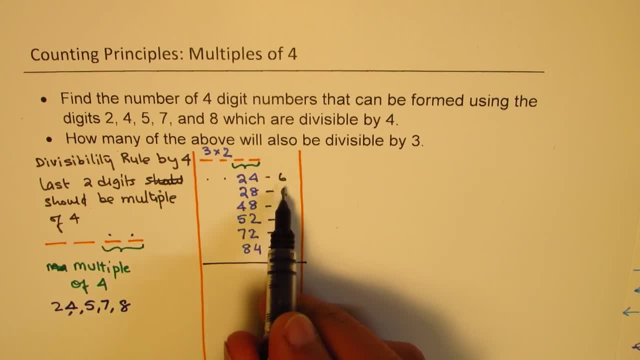 so the answer here is 1, 2, 3, 4, 5, 6 of 1, 2, 3, 4, 5, 6, so 6 times 6, which is 36, right? so we have 36 numbers. so we have 36 numbers of four digits as multiple. 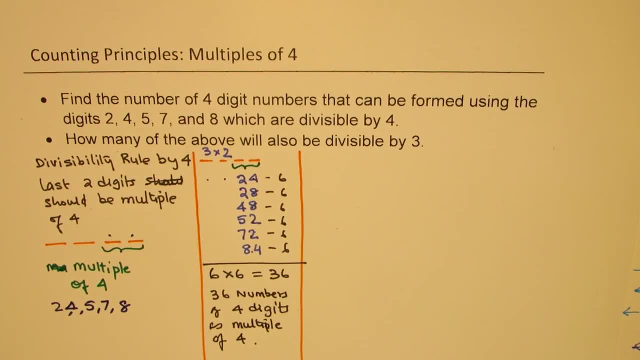 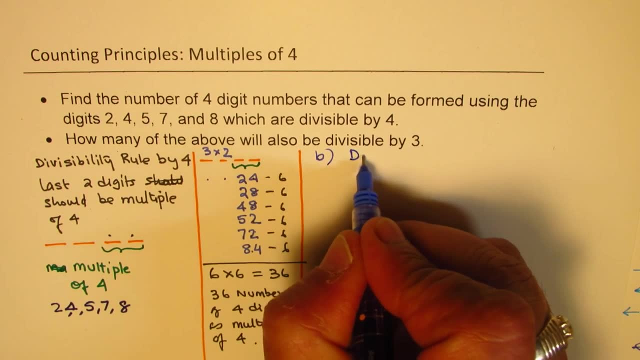 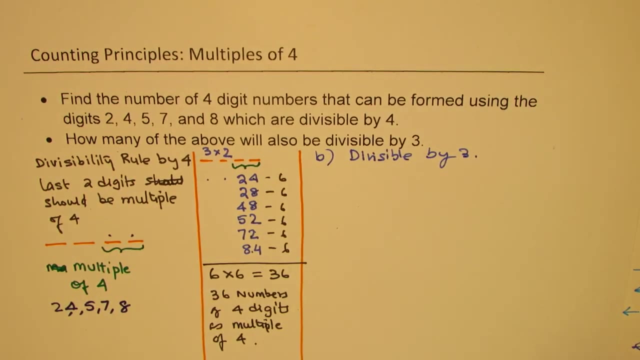 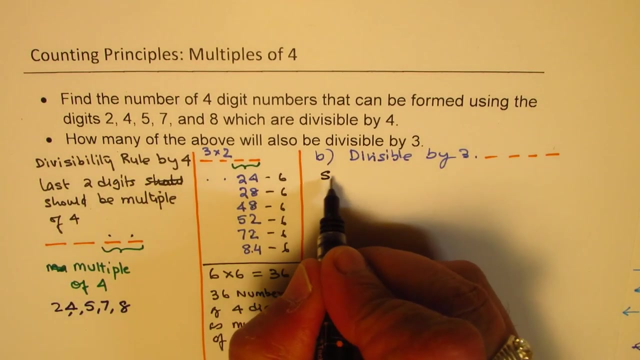 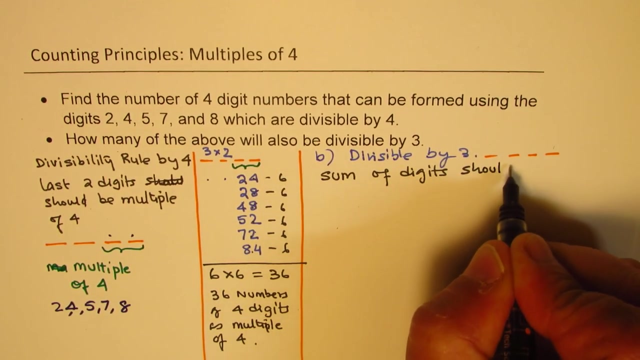 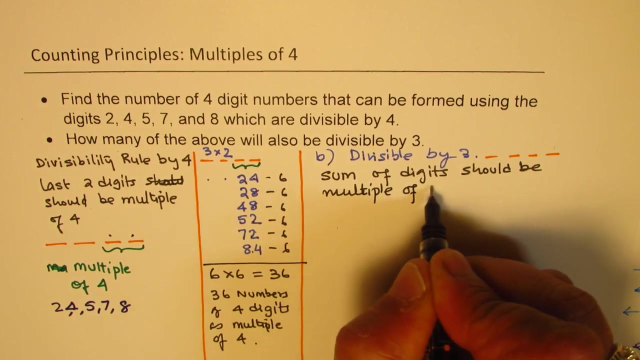 of four clear. so that is how we are going to solve this part. now let's look into part B, which is divisible by 3. now, what is the rule for that? so if you are taking these four digits, in that case sum of digits should be multiple of three. that is the rule, right? so that is the rule. now we know we have. 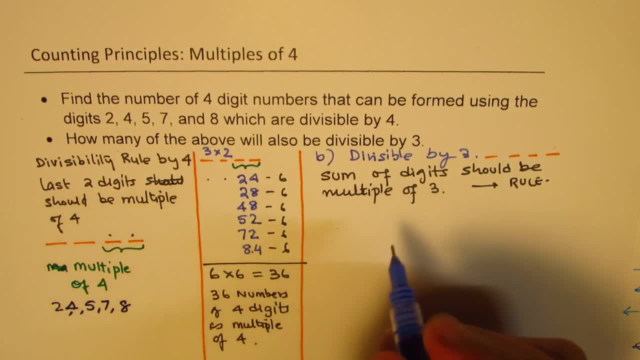 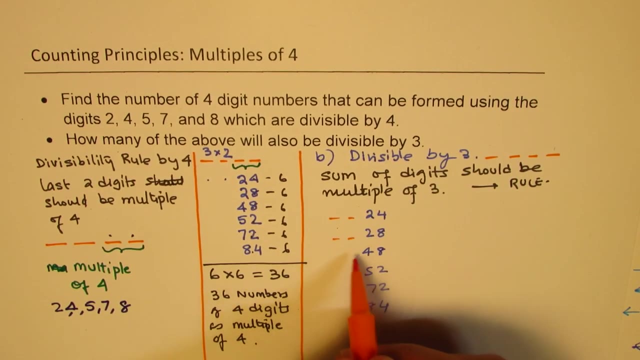 to select out of these. so let's again consider these numbers. so we are ending with 24, we are ending with 28, with 48, 52, 72 and 84. now we have two more positions to fill. what could be these numbers which could give us addition, which is a? 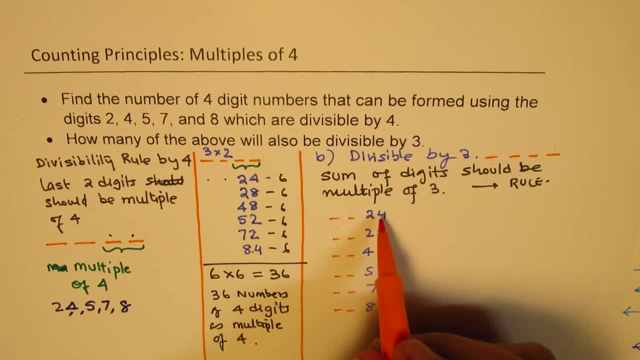 multiple of three. now, two plus four is six, right, so we already have a multiple six. so these two, we are looking for multiple of three and we have a choice between these numbers: two, four. so we have to now look into back to this right now. so if I have engaged two and four, we are left with five. 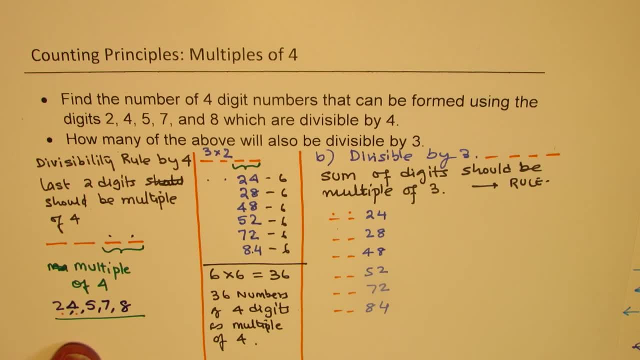 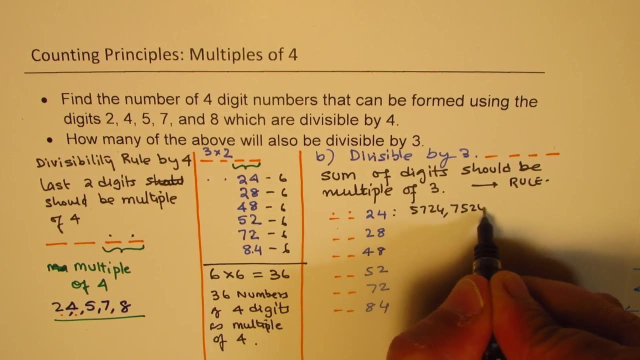 seven and eight. so what numbers could be formed, ending with 24. so five and seven is twelve. seventy five and fifty seven can work right. so five, seven, two, four is okay. similarly, seven, five, two, four is also good enough. so these are combinations which will give you addition five plus seven, twelve and thirteen. 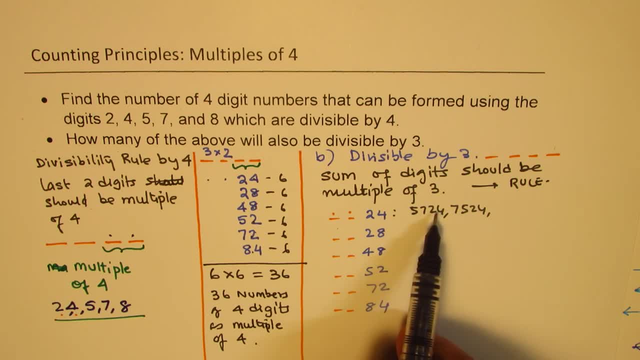 fourteen and four eighteen, which is a multiple of three, three times six. correct likewise. so what is? is there any other combination? can we do eight and seven? yes, we can. eight plus seven is fifteen, right, so we could have 87, 24 and 78, 24 also. so, as you can see, we have. 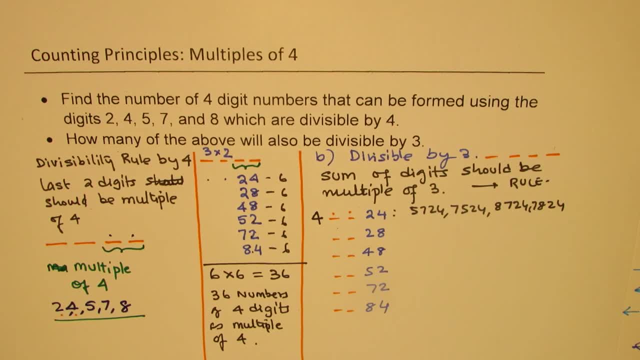 four combinations. right, these are the four numbers, is that okay? right now, let's look into 28. 28 is ten, so if we take away twenty eight, we're left with these. so ten plus what? four and five is nine. that is not far. and seven is eleven. ten plus eleven is: 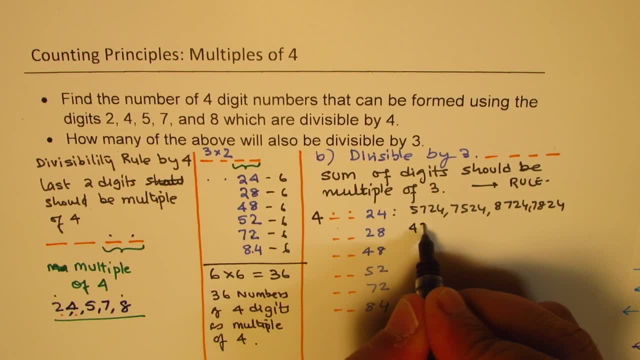 21. that works. so we have 47,, 48,, 28, and 74, 28. that is one possible. now. eight and five is 13 plus 10 is 23, which doesn't work. so these are the only two numbers we get: 248, 4 plus 8 is 12. 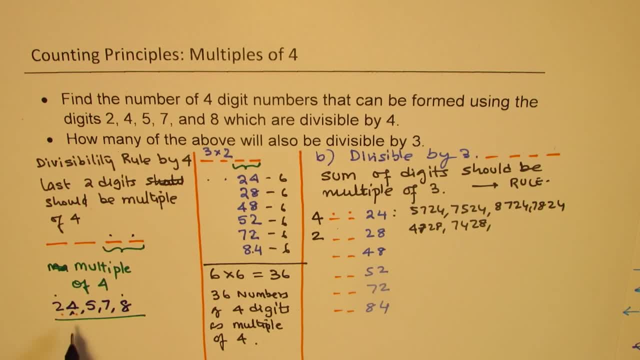 okay, so 12 even. it evens out multiple of 3 now in these 7 and 5 is 12, it works. so we get 7, 5, 48 and we have 57, 48. okay, 75 works. so for 2 and 7 also works right. so we have 27, 48 and 72, 40, that also. 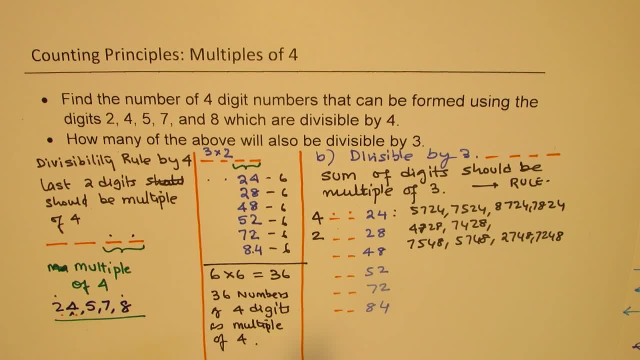 works right. so that also work. so these are the four numbers which can work. so we have four combinations. fifty two, five plus two is seven. so if I take away fifty two, seven and six, 7 and 4 is 11, 7 and 11 is 18, that works. so we have got 74, 52 and 47, 52. okay, 7, 5 and 2 is 7. 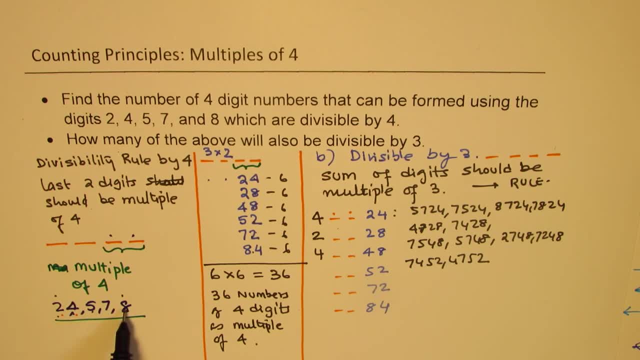 okay, if i take 4 and 8, that will not work. 8 and 7, 15, that will not work. so these are the only two combinations. if i take 72, 7 and 2, which is 9, 3 times 3, so we're looking for 4 and 5, 5 and 4, that